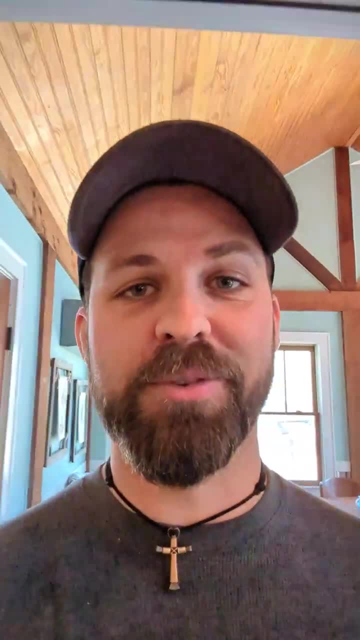 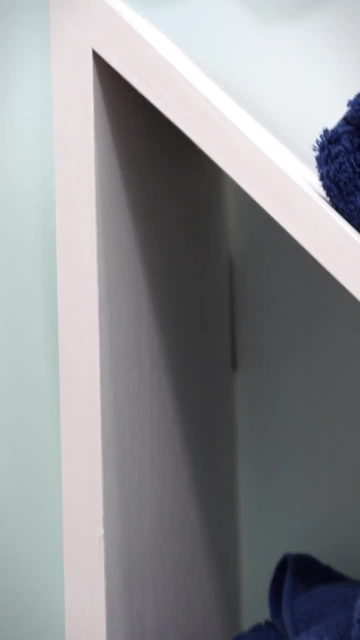 I remember taking geometry in high school and thinking: man, I ain't ever going to use this stuff. You're going to learn today. We made this modern looking shelving and I had to bust out the old trig knowledge to figure out the sizing and cut angles. And I'm going to show you a cool app. 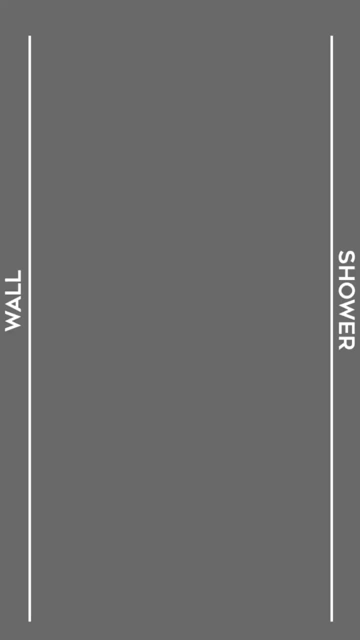 that takes all the thinking out of it. We have a space between a wall and a shower that we want to install this shelving, And we know that the width of this space is 25 inches wide. We want the shelving to fill the majority of the space, So we'll design it to 24 inches wide to leave a 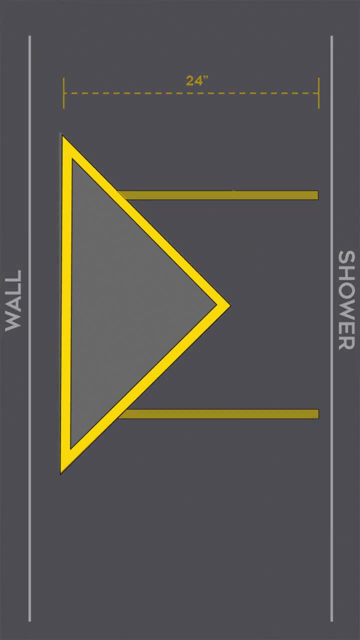 little bit of wiggle room. I somewhat arbitrarily chose for the large triangle here to be half of the overall width, So 12 inches. now, because this is a right isosceles triangle and we know this dimension is 12 inches, This dimension has to be 24 inches, trigonometry, bro. So now that I got, 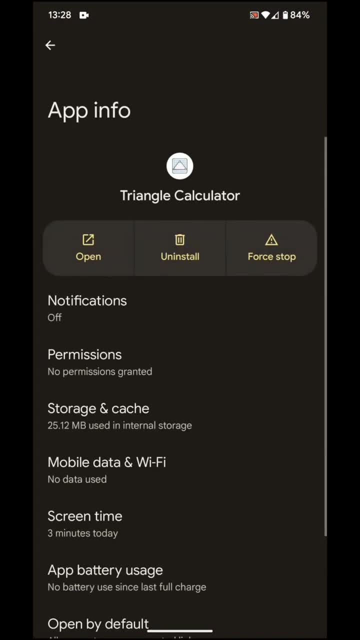 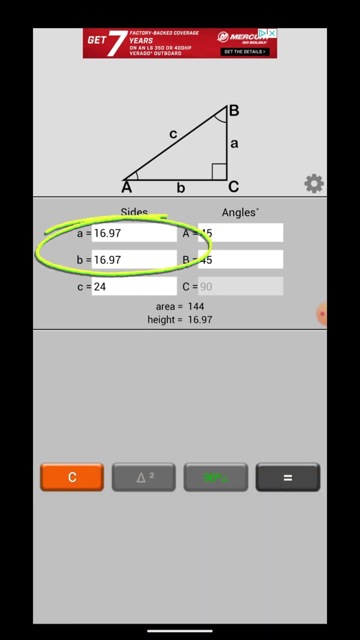 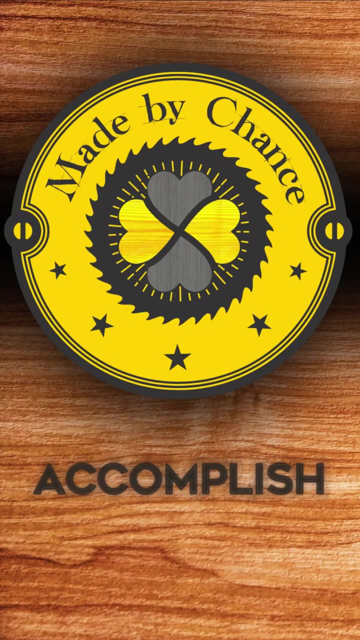 these dimensions and angles. I can bust out my handy dandy app here called triangle calculator, which I'll link in the description, And I can actually use it to calculate the two missing dimensions that I need. Thanks for watching. 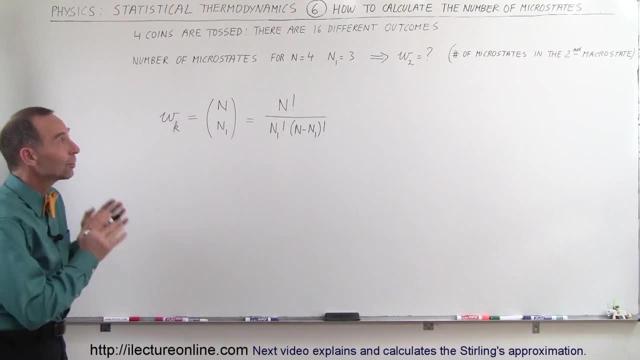 Welcome to ElectronLine. and now let's go take a look and see how to calculate the number of microstates in thermodynamic, statistical thermodynamics. So here again we're going to start out by using a simple experiment where we have four coins. we're going to toss the four coins. 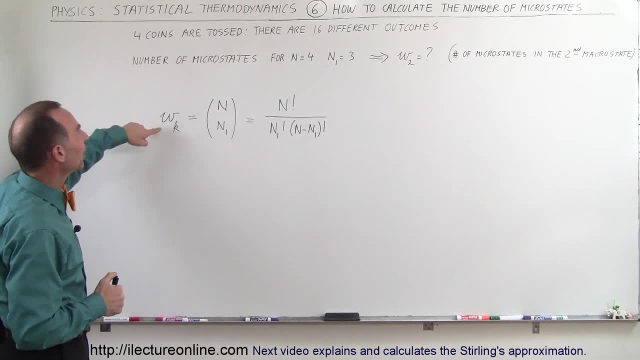 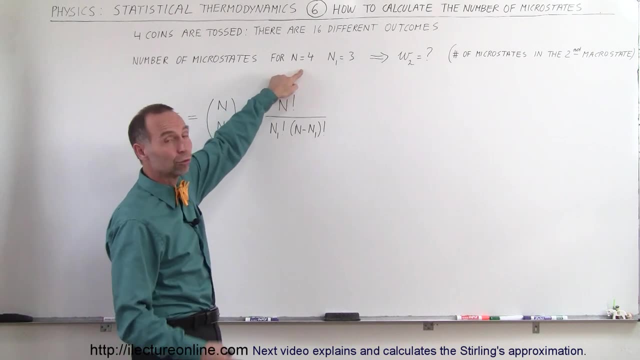 you can have 16 possible outcomes and we're going to find the number of microstates in, let's say, the second microstate. We're going to have the situation where n is equal to 4, there's four entities, four coins. n sub 1 equals 3,. 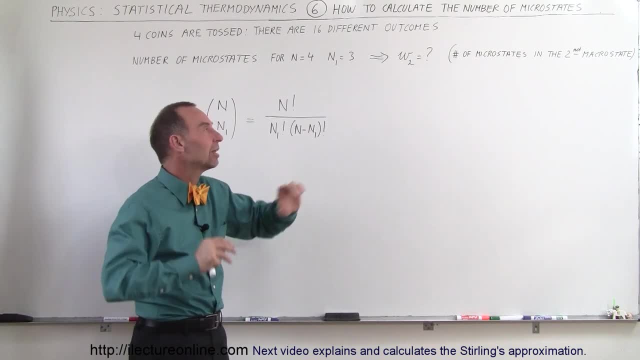 meaning the number of heads in a particular microstate is equal to 3, which means we're talking about the second microstate. Remember, the first one had four heads, the second one had three heads, the third one had two heads, and so forth. 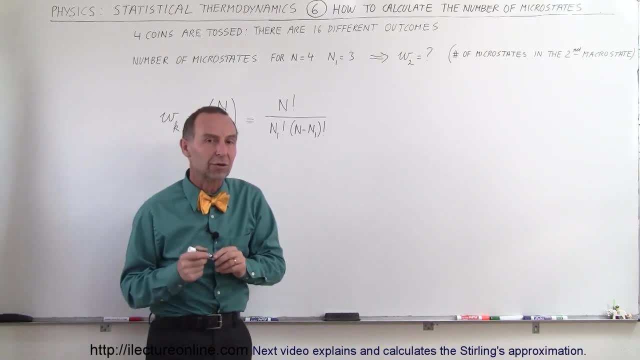 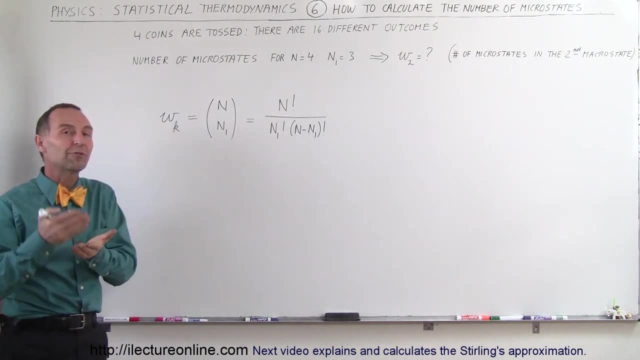 So we're looking for the number of microstates in the second microstate. Alright, here's a general equation: W sub k, remember, W represents the number of microstates, k represents the microstate that we're concerned on that we well, let me put it again this way: